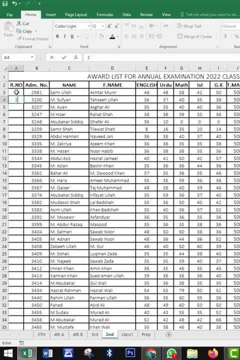 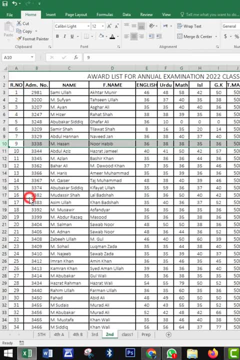 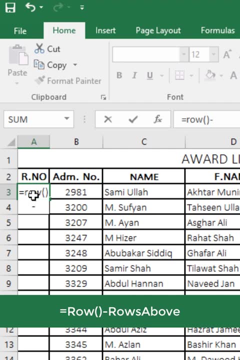 If you fill serial number column in Excel with a traditional flash fill option, your data could mess up if you delete some rows from your data. Here is a more efficient way to fill serial number column in Microsoft Excel. Click in the first cell of the serial numbers, Enter this formula and hit enter. 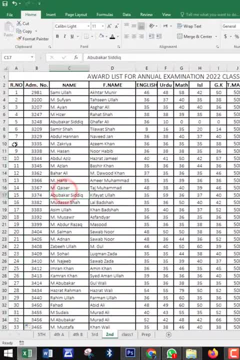 Now, if you delete one or more rows, the serial number will be automatically adjusted. Great isn't it. 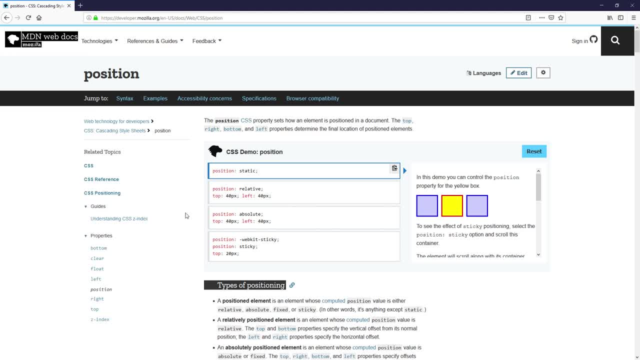 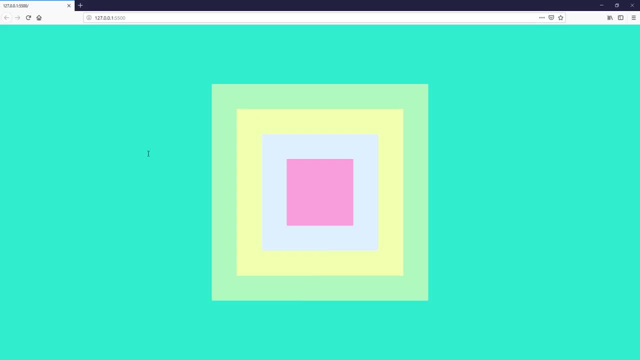 Absolute and relative positioning is one of the most basic things in CSS that everyone knows, But do you really understand how they actually works? In this video, we're going to talk about absolute position versus relative in details, along with some examples. Let's check it out. 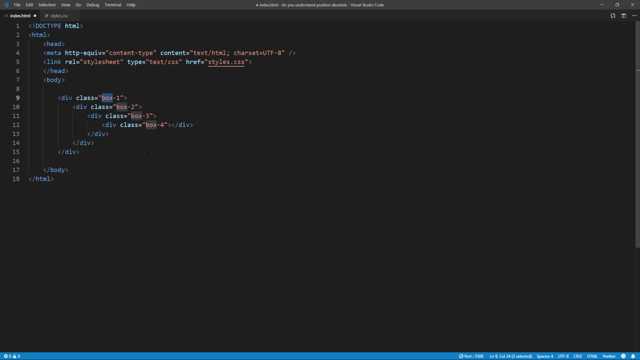 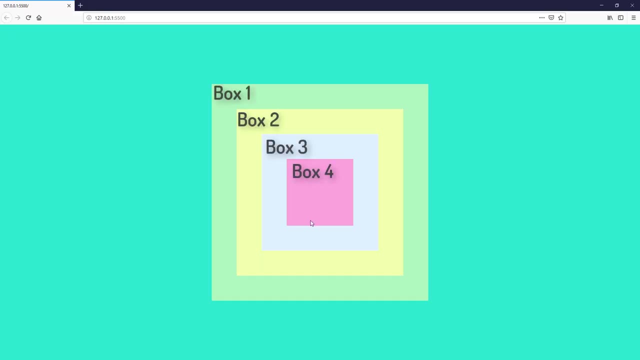 So here is our example page. I have four boxes: Box 1 is parent of box 2,, 2 is parent of 3, and 3 is parent of 4, respectively. I only set the size and background, then use this play flex to center them. 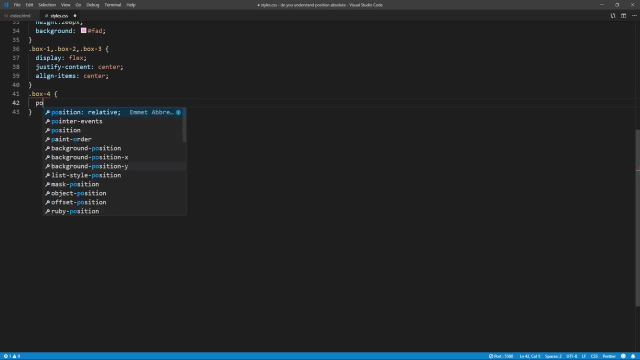 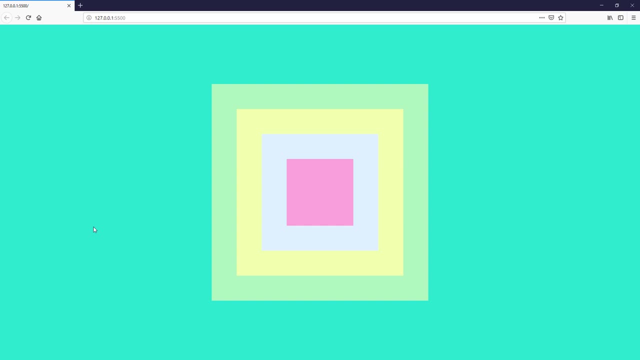 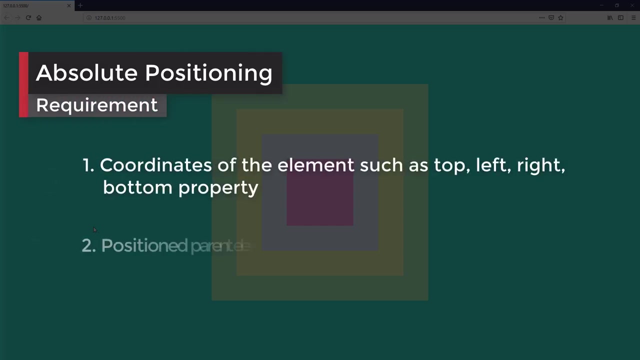 Now I'm going to try setting the position of box 4 to absolute. You see that nothing happened. This because an element need two things to position itself. First is the coordinates, such as top, left, right, bottom properties, And second is the parent element it can position itself to. 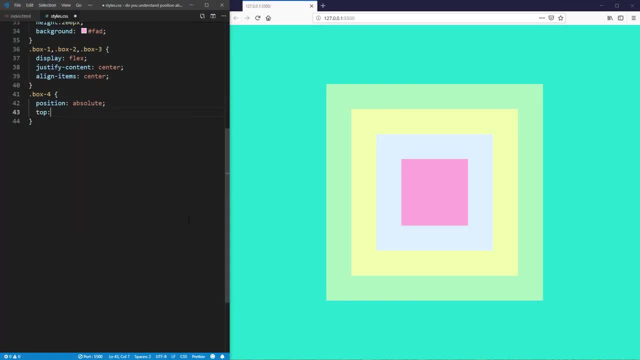 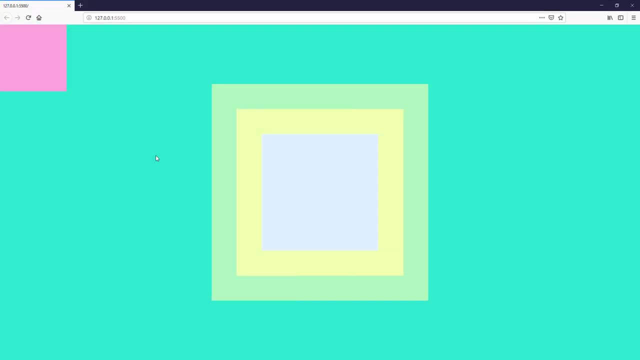 So now I'm going to try setting top left to 0.. You will see that the box 4 is now positioned itself to the body instead of top left corner of box 3.. This because, in order to be an eligible positioning parent, the elementos.